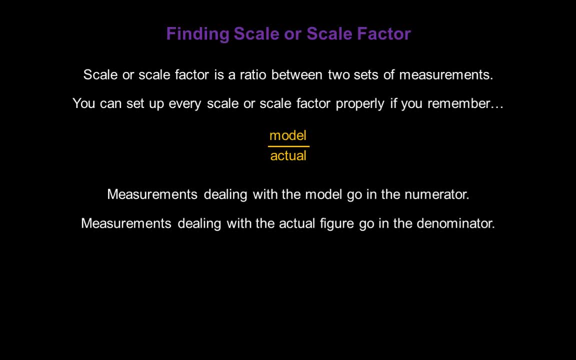 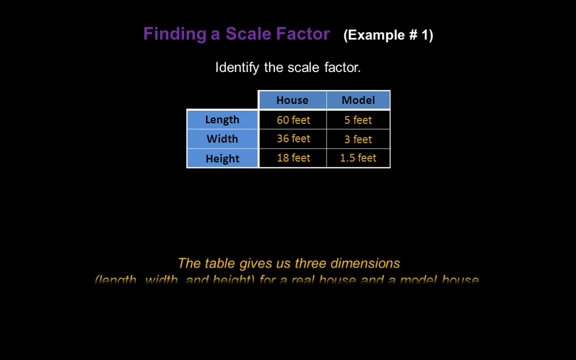 Measurements dealing with the actual figure always go in the denominator. Now take a look at this table and let's identify the scale factor. The table gives us three dimensions: length, width and height for a real house and for a model of that same house. 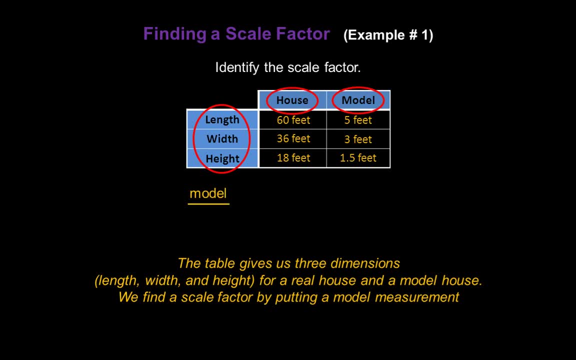 We find a scale factor by putting a model measurement over the same measurement on the actual object, Model over actual. Since all dimensions of our model and actual object will be proportional, we could use any one of these three dimensions to find the scale factor. 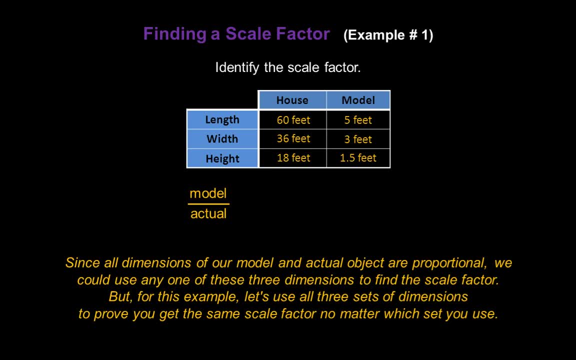 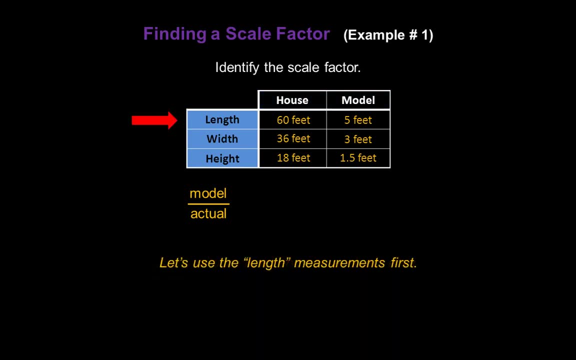 But for this example let's use all three sets of dimensions to prove you get the same scale factor no matter which set you use. Let's start by using the length measurements first. Put the model measurement, the five feet, over the actual length of sixty feet. 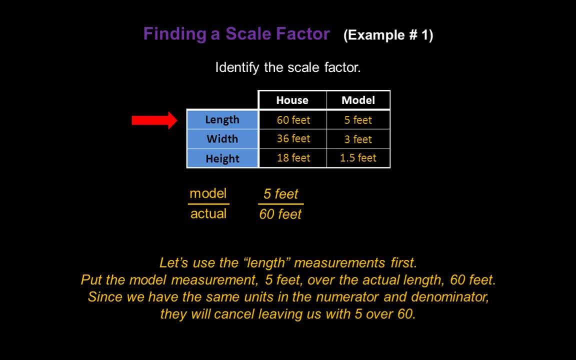 Since we have the same units in the numerator and denominator, they're going to cancel, leaving us with five over sixty. But five over sixty can be reduced. We can divide both numbers by their common factor of five. So let's divide the numerator and denominator by five. 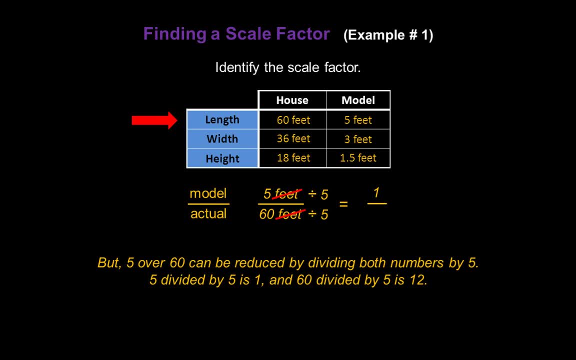 Five divided by five gives us one in the numerator, and sixty divided by five gives us twelve in the denominator. So our scale factor is one. twelfth, Now let's use the width measurements and see if we get the same answer. Put the model measurement, the three feet. 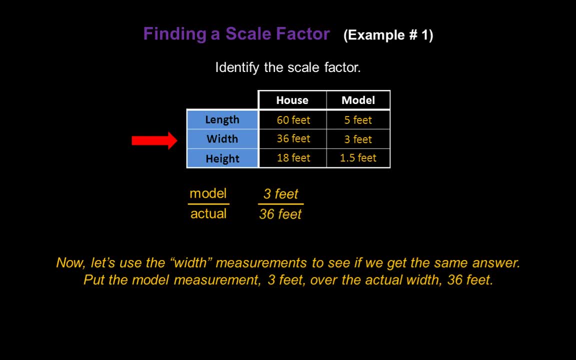 over the actual width of thirty-six feet. Again, we have the same units in the numerator and denominator, so they're going to cancel, leaving us with the numbers three over thirty-six. But three over thirty-six can also be reduced by dividing both numbers by three. 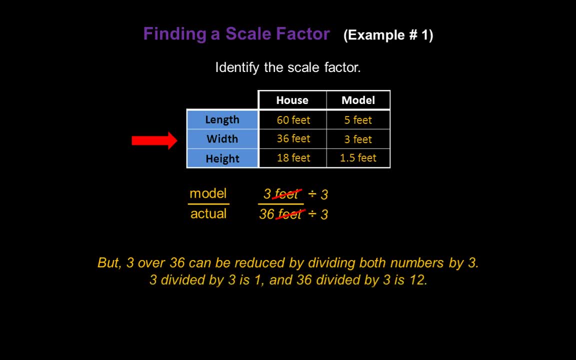 So let's divide the numerator and denominator by three. Three divided by three gives us one in the numerator, and thirty-six divided by three gives us twelve in the denominator. So our scale factor is the same one. twelfth, as we expected, 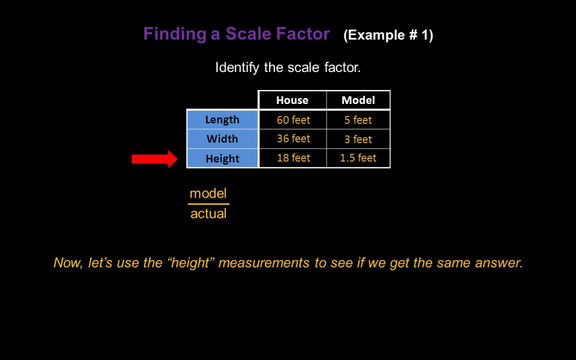 Finally, let's use the height measurements and see if we get the same answer Again. put the model measurement one and a half feet over the actual height of eighteen feet. Again we have the same units, numerator and denominator. so they're going to cancel. 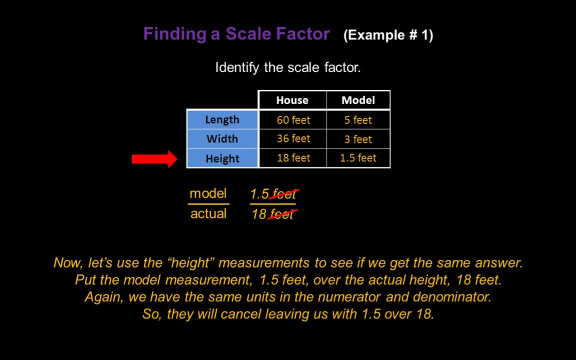 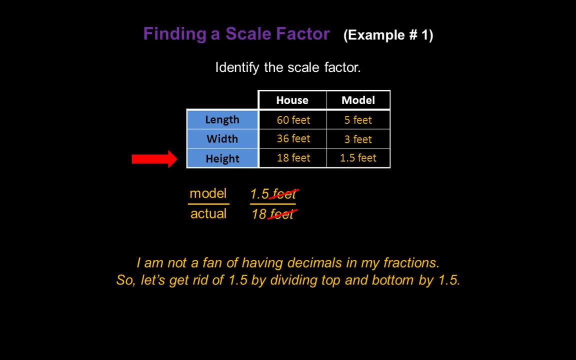 leaving us with the numbers one point five over eighteen. Now I'm not a fan of leaving decimals in my fractions, so let's get rid of one and a half feet by dividing top and bottom by one and a half. When we do that, one and a half divided by one and a half. 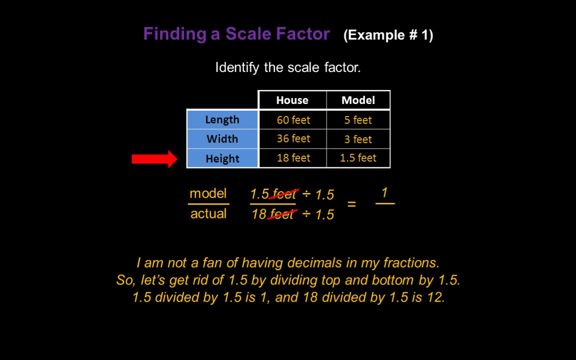 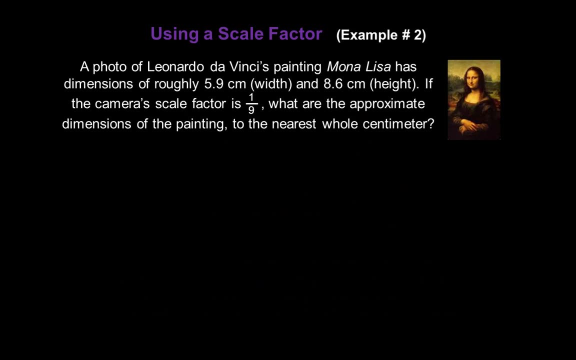 becomes one in the numerator, and eighteen divided by one and a half is twelve. So again, our scale factor is the same one. twelfth, as we expected, A photo of Leonardo da Vinci's painting Mona Lisa has dimensions of roughly the same. 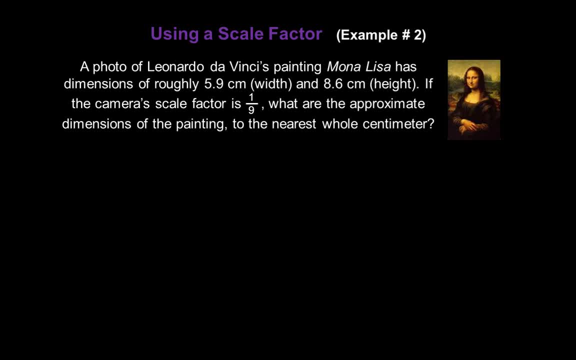 approximately five point nine centimeters in width and eight point six centimeters in height. If the camera's scale factor is one ninth, what are the approximate dimensions of the painting to the nearest whole centimeter? Now we have to perform two separate calculations here. 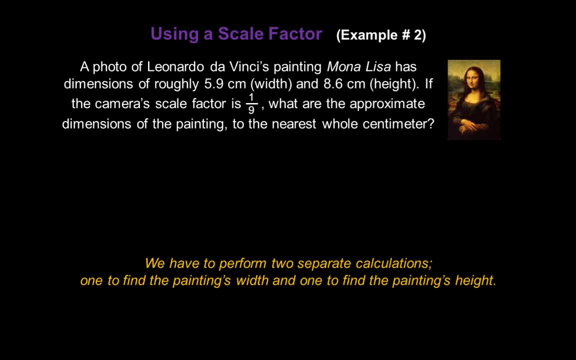 one to find the painting's width and one to find the painting's height. The painting is the original or actual object and the photo of the painting is the model. Now remember our scale factors are set up as model over actual. 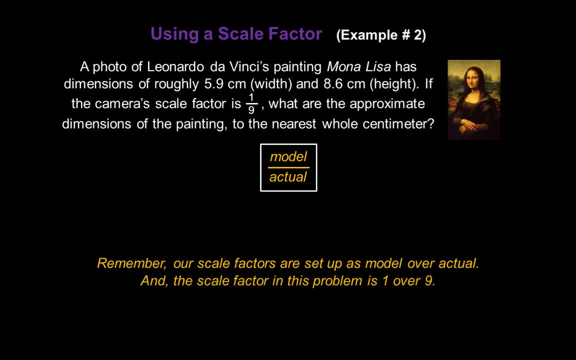 so I'll write that down so we don't forget it. And the scale factor in this problem is one over nine, so that's going to be one of our ratios. Now we can set up proportions using the dimensions given and this scale factor. 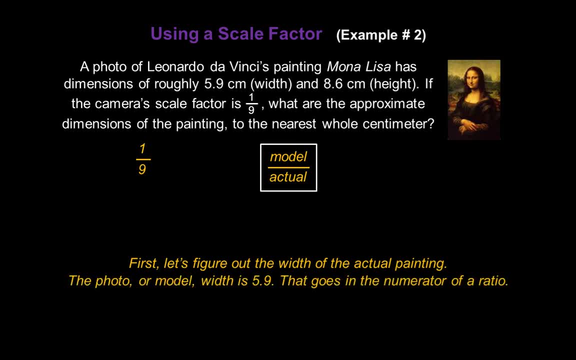 First let's figure out the width of the actual painting. The photo or model width is five point nine, So that's going to go in the numerator of our second ratio. So we'll have five point nine in the numerator And we're looking for the actual width. 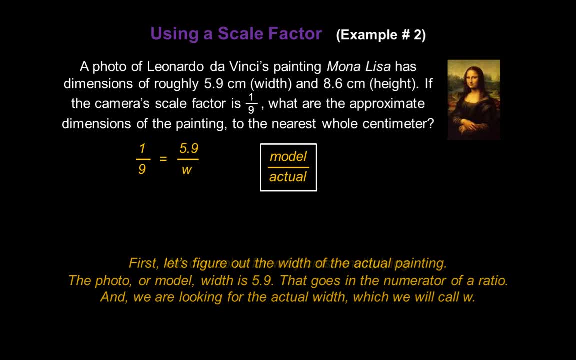 so let's go ahead and call that W in the denominator. Now we can solve for W by cross multiplying: One times W is W, and nine times five point nine is fifty three point one Now, since we're supposed to round to the nearest whole centimeter, 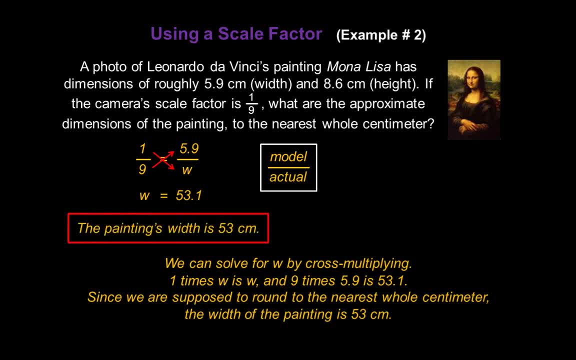 we'll say the width of the painting is fifty three centimeters. Now we use the same method to determine the painting's height. Again, start with our scale factor of one over nine. That's going to be one of our ratios in the proportion. 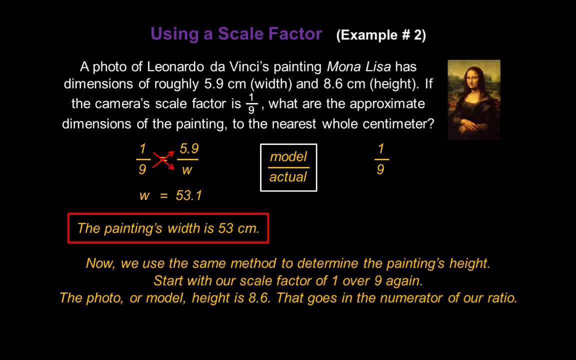 The photo or model height is eight point six, and that goes in the numerator of our second ratio. We're looking for the actual height. Let's go ahead and call that H for height. Now we can solve for H again by cross multiplying. 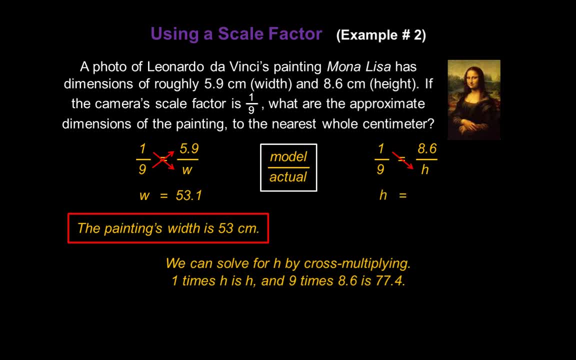 One times H is H and nine times eight. point six is seventy seven point four, Since we're supposed to round to the nearest whole centimeter, the height of the painting is seventy seven centimeters. On a map, the distance between Portland Oregon and Eugene Oregon. 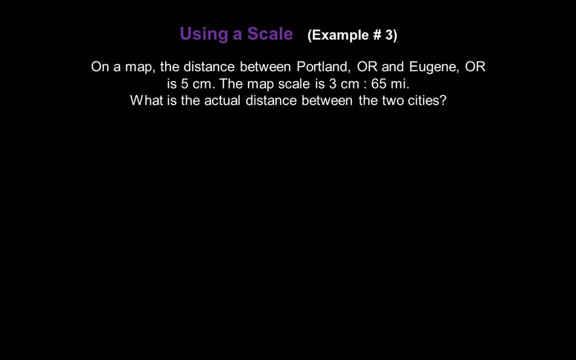 is five centimeters, The map's scale is three centimeters equals sixty five miles. What's the actual distance between these two cities? Well, we need to set up a proportion to solve this problem. Remember, we always set up our ratios as model over actual. 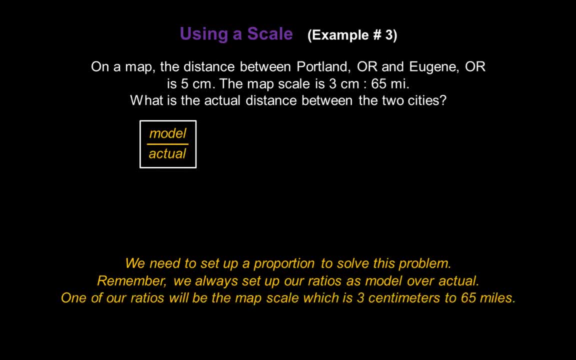 so let's write that off to the side so we remember it. One of our ratios is going to be the map's scale, which says it's three centimeters to sixty five miles. Now the only other number we have in this problem is five centimeters. 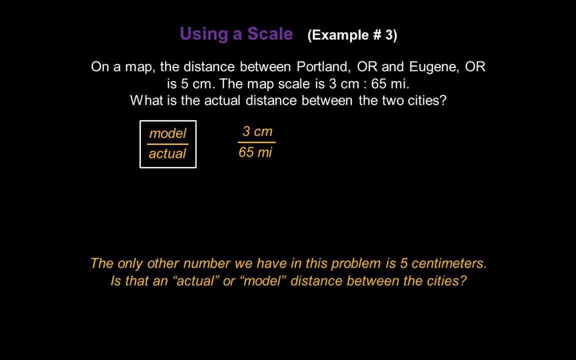 What do we do with it? Is that an actual or model distance between the cities? It's a distance on our map, so it's the distance on a model. That means five centimeters goes in the numerator of our second ratio. Another way we know that the five centimeter number has to go in the numerator.